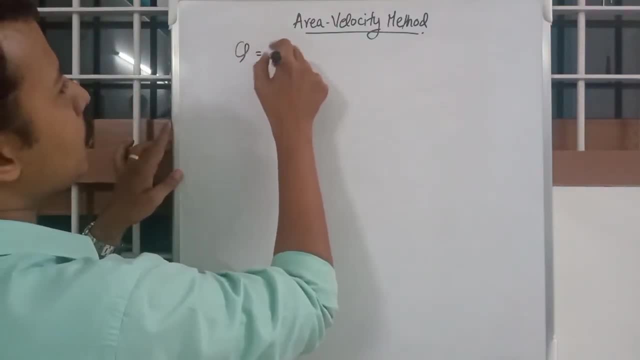 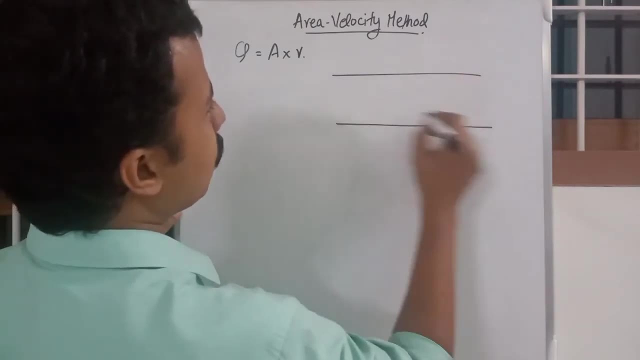 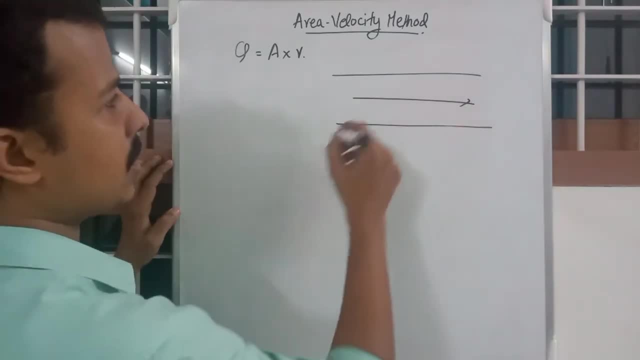 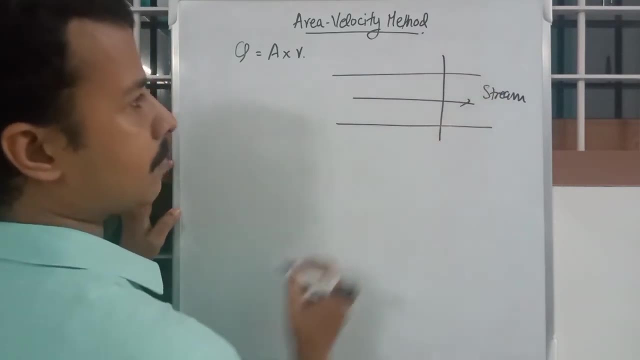 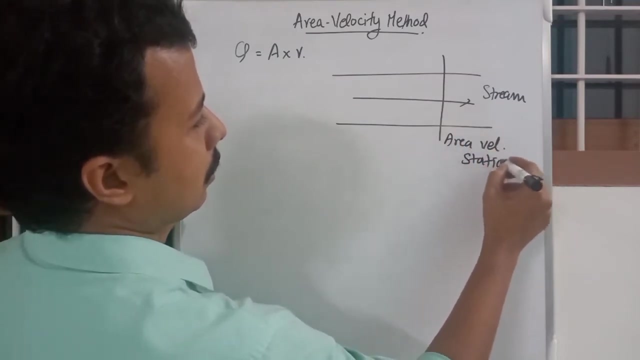 So if suppose this is a flow, This is flowing water flow, stream stream is flowing in this direction, This is a stream. okay, We will be taking a particular section and this section is known as area velocity station. okay, So we cannot measure all the sections. 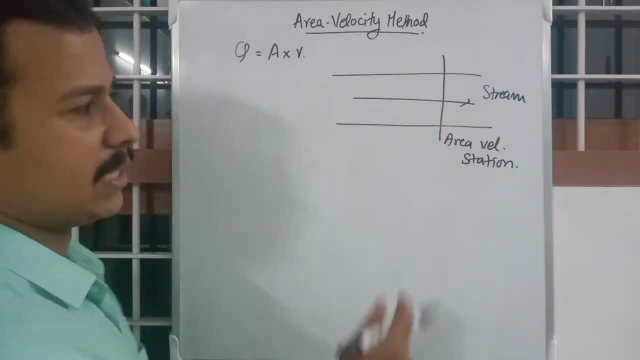 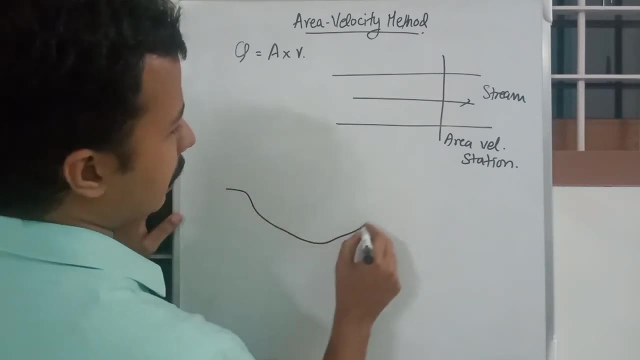 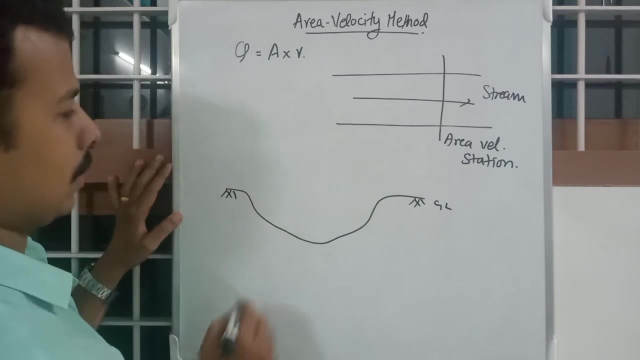 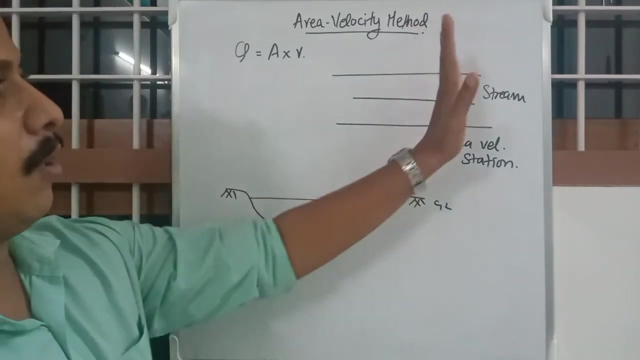 We will be selecting one particular most suitable section and we will call this area velocity station, station as a section, and that section will be somewhat like this: suppose this is the ground level, okay, and this is the flow of water. suppose current flow of water is this: this is the section of this stream, okay, what we are going to do, 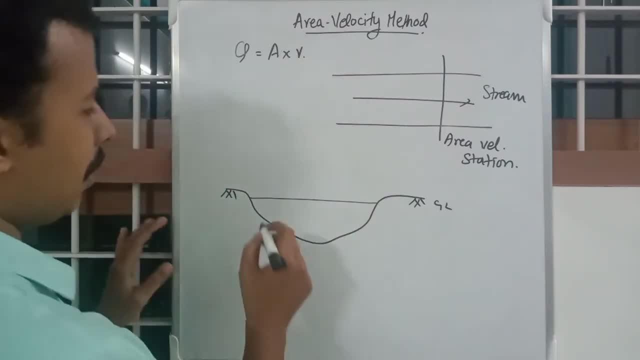 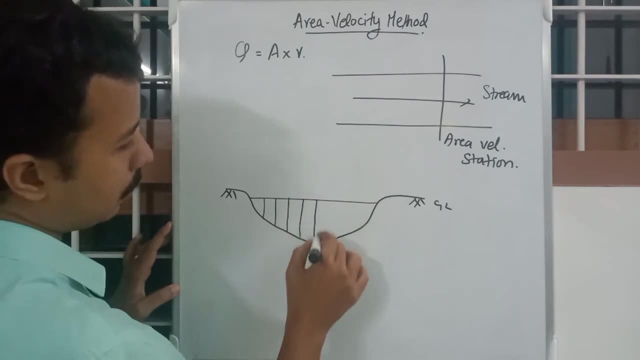 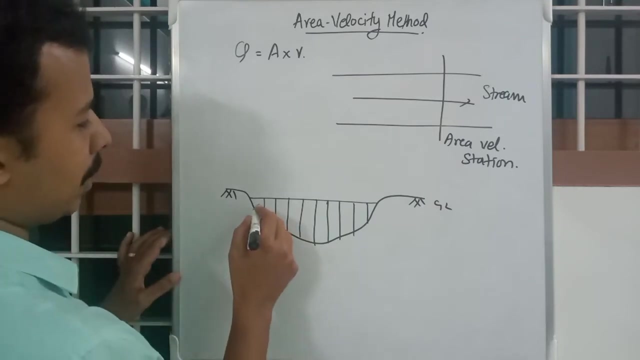 in an area. velocity method is very simple. we'll divide all this section into small parts, okay, and we'll number it or name it: one, two, three, four, five, six, seven, etc. and most probably this distance will all be equal, maybe one meter or 0.5 meter, according to our size of stream and quantity of flow of water to 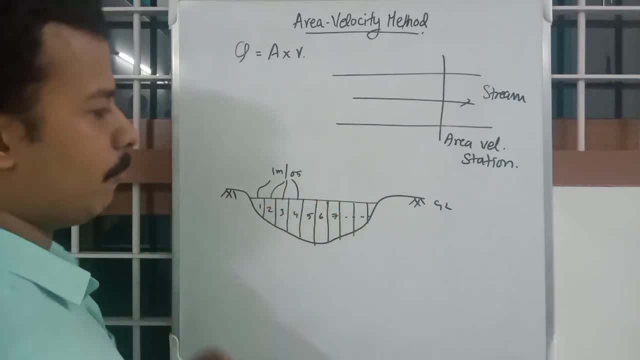 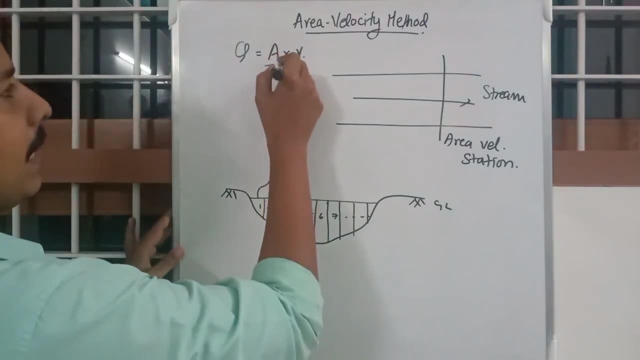 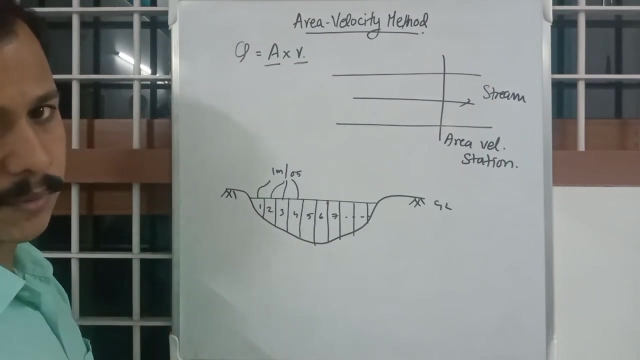 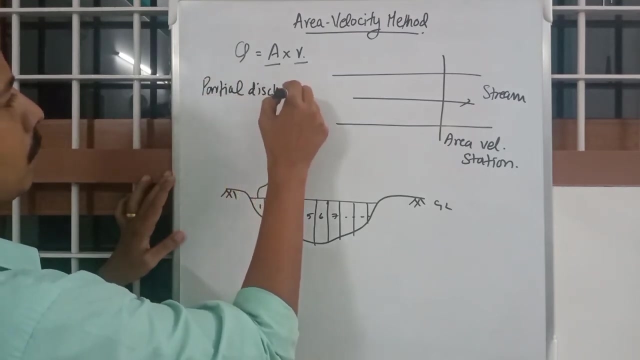 be so. all this will be equal values and, considering each section separately, we will calculate area from section diagram and then, for each section, we will calculate velocity, the. hence we will calculate partial distance in terms of volume, if you will now, if we communicate a equation of the partial 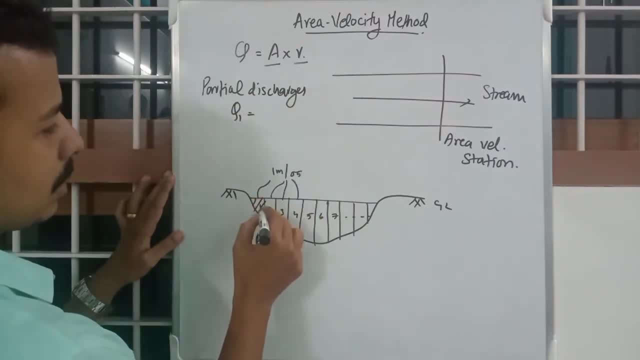 distance. here you take the state of the volume, okay, so you write down the place of the volume, Grassok, and one point of the volume of water known as temperature. so, temperature of these twoENA. this is our time and this will be the time for these twooutro spielen these two different. 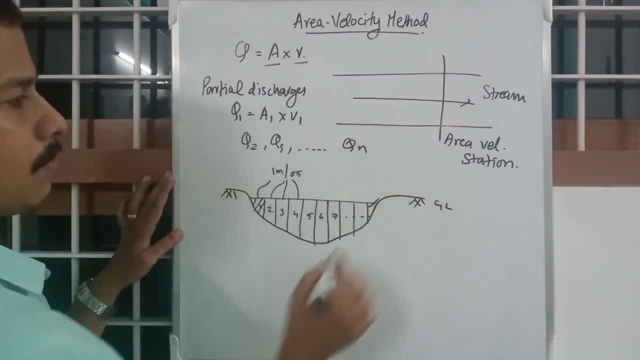 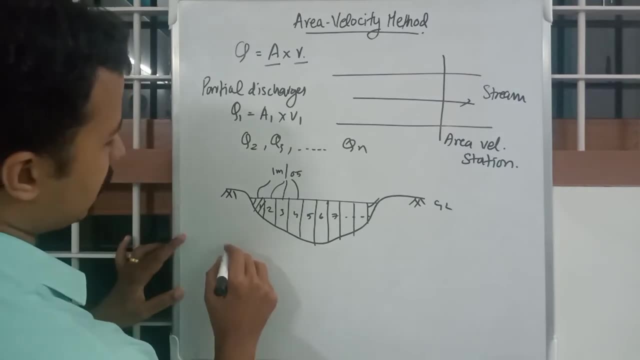 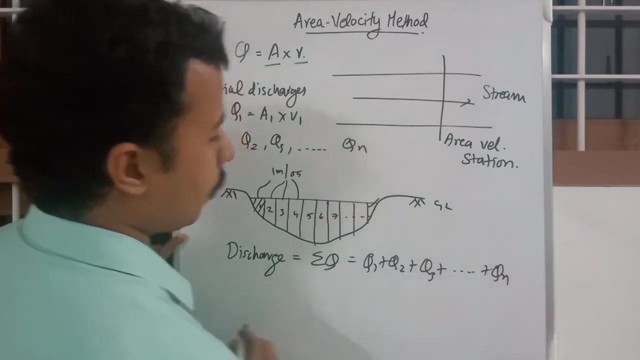 points if we want to know. what does this mean in terms of other是什麼? finally, what it involves the system, because, but in these two of these, now you, the discharge will be equal to sigma q, that is, q1 plus q2 plus, q3 plus, etc. qn. 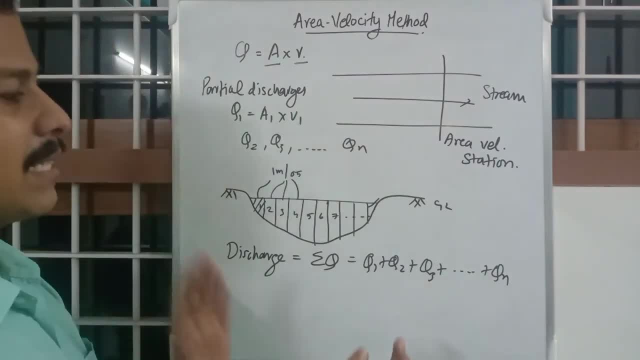 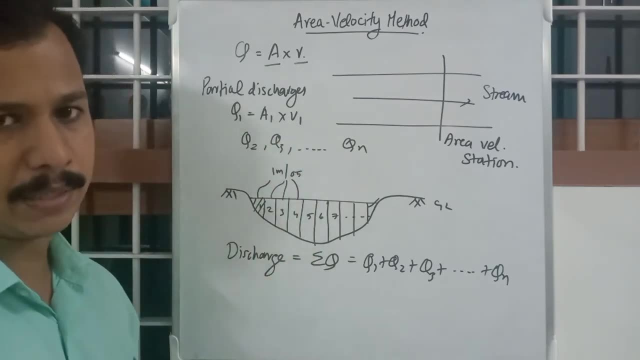 ok, so summation of all the partial discharges will give you the total discharge, and by total discharge we got stream flow measurement. ok, that is concisely, briefly, the concept of area velocity method. ok, so this area measurement can be done very easily by- if you get the cross section of that. 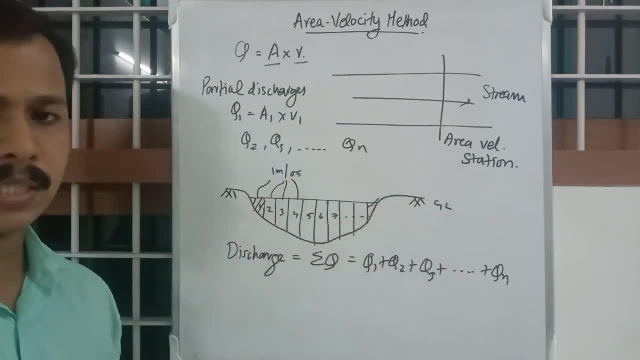 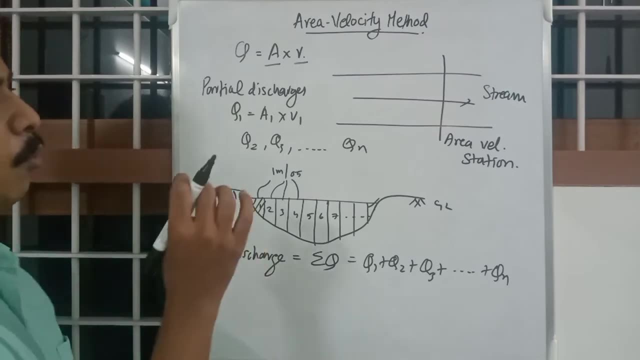 stream or this velocity area station, you get the cross section. you can measure it from a map or you can measure it from a section itself, manually, directly. ok, then how do you calculate the velocity, or how do you calculate this velocity? for this we have a number of methods. first one is floats. 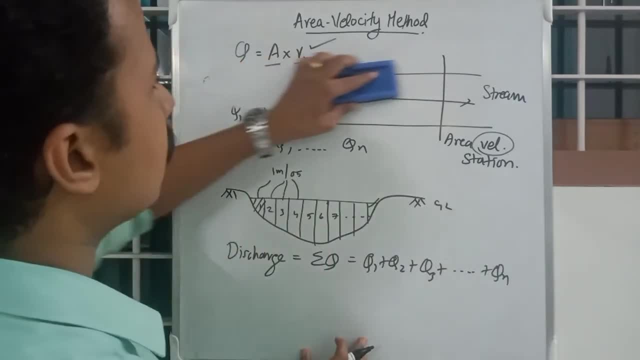 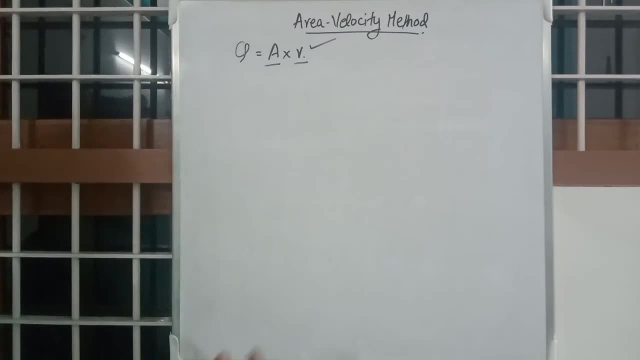 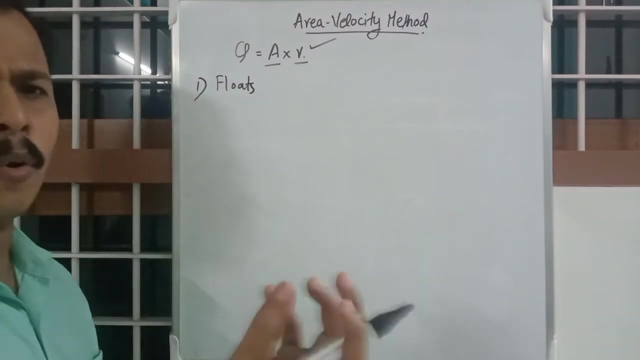 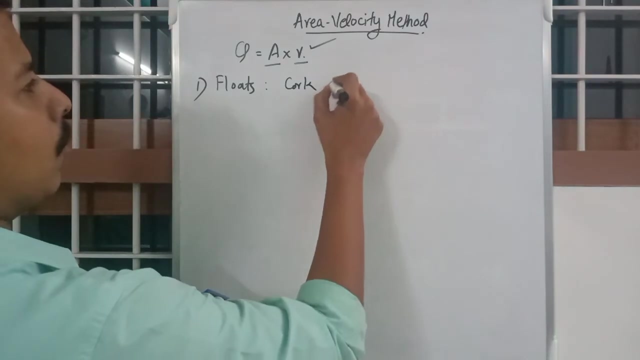 floats, as the name indicates. again, it's just the any floating substance. maybe it's a cork, maybe it's a very big, appreciable amount of paper, any material that floats on water. most probably we will be using a cork or paper, etc. paper, roll of ball of paper. 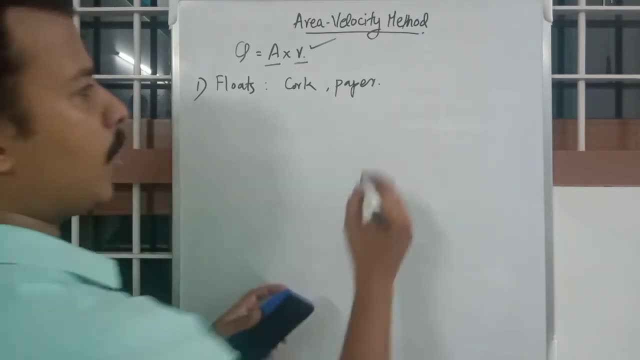 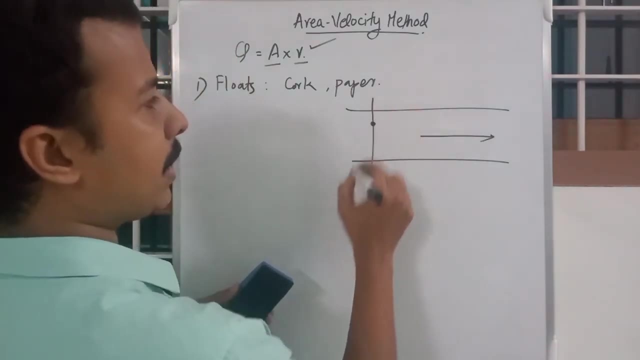 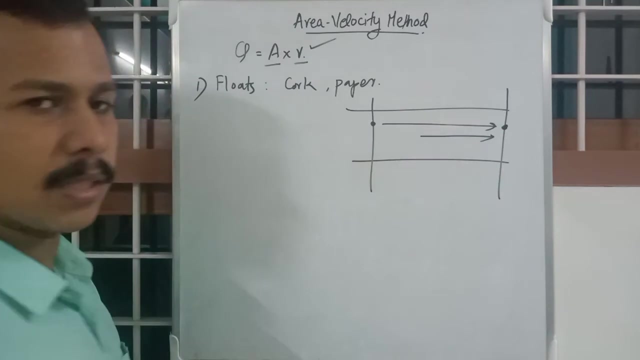 etc. all these things can be considered as float. what we will be doing is, if this is the stream going this side, we will drop the float in here and measure the time taken for the float to reach there. ok, so we know the distance. say, for example, we know the distance. 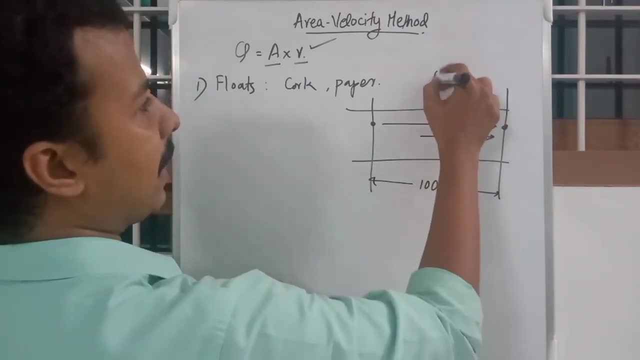 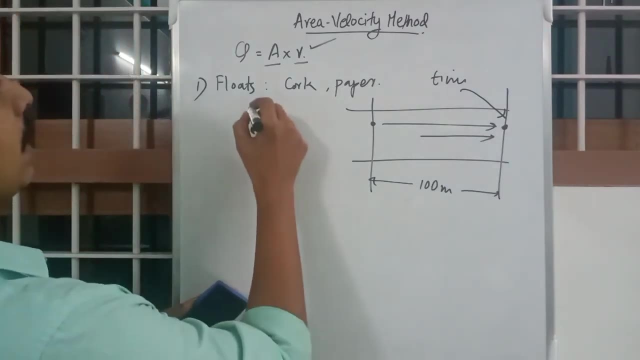 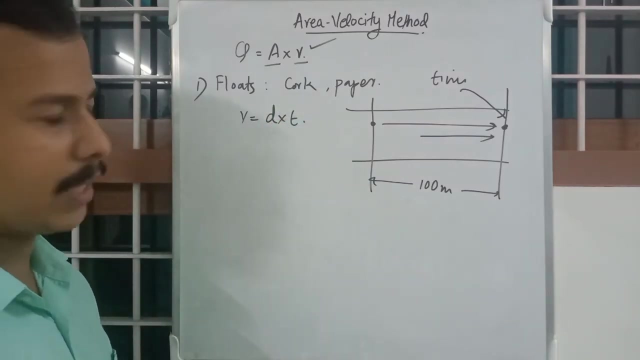 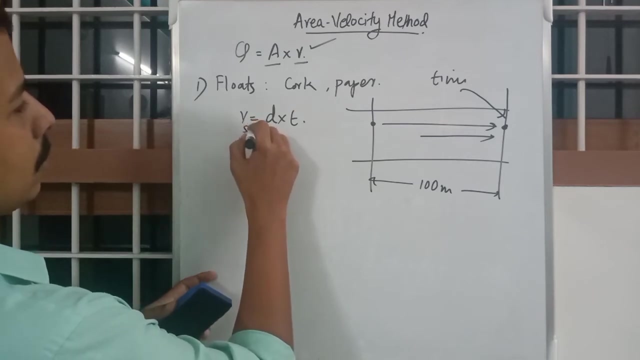 of y or it may say 100 meters, and we have the time measure with the stopwatch to reach here. so velocity will obviously distance into time. you can you get very easily, but this velocity you get will be surface velocity, ok, as it is only floating like this. 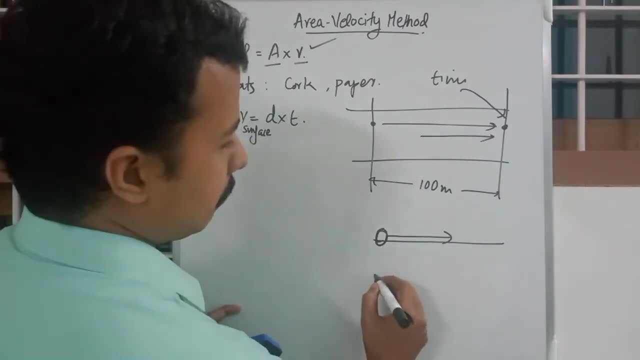 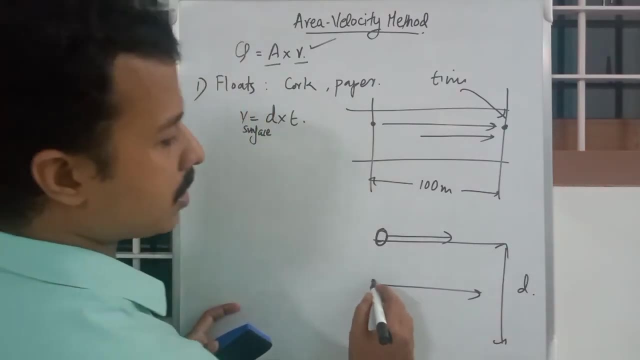 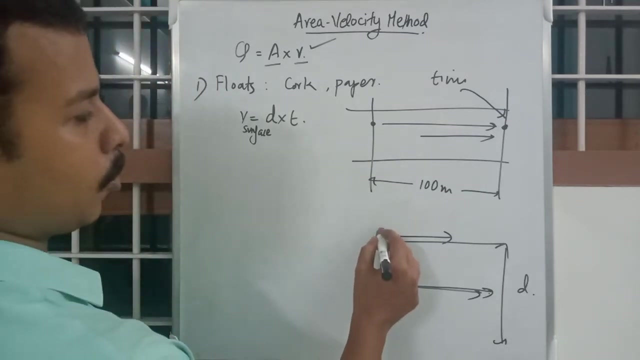 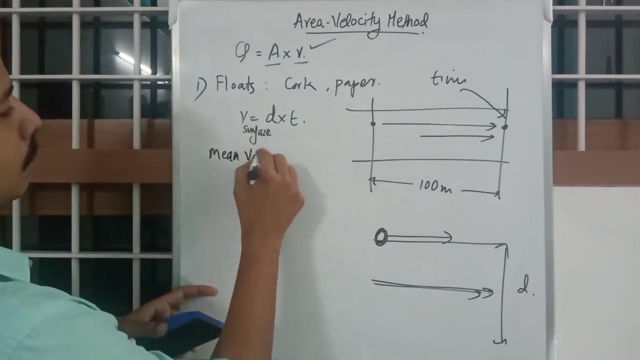 ok, but mean velocity will be somewhere in the middle if this is the depth of stream mean velocity. if you want to measure the mean velocity, it will be somewhere in the midpoint of the depth, but we will be by floats, will be measuring it on the surface only, so to get mean velocity you multiply this: 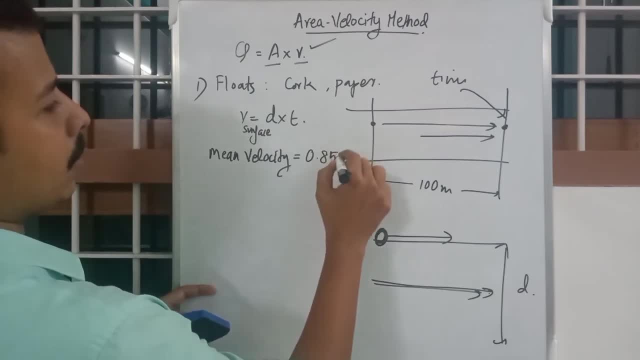 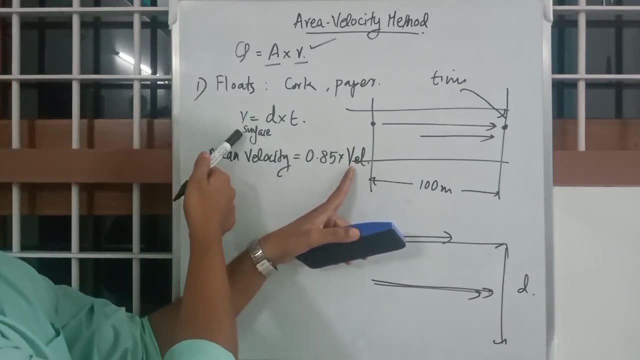 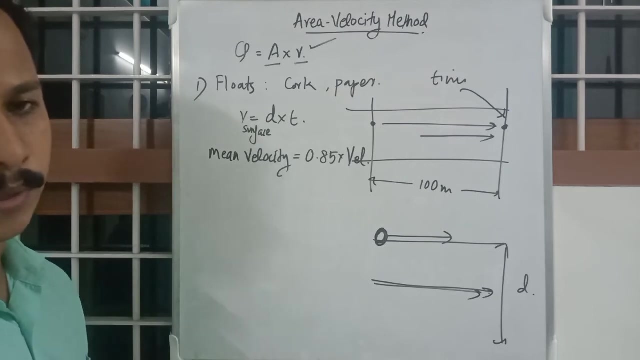 velocity into 0.5, the velocity we got from the surface float will multiply with 0.5 to get mean velocity of stream. ok, that is one way to do or to measure velocity of a stream by floats. there is one more time: some surface floats. 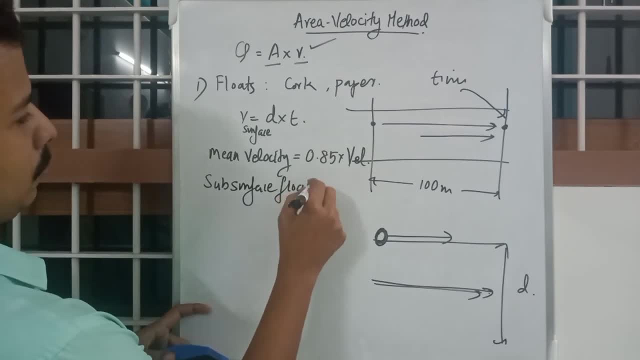 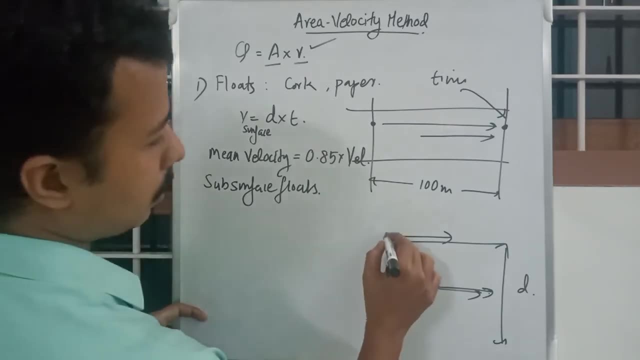 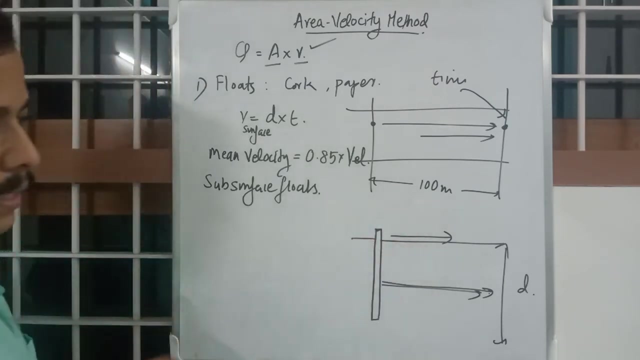 subsurface floats. they are a road example. this is a road, ok, this wooden road, made specifically to keep submerged or float vertically. it is a wooden road. if you dip in the water, if you throw it in water, it will be suspended, floated vertically. ok, like this and the same. 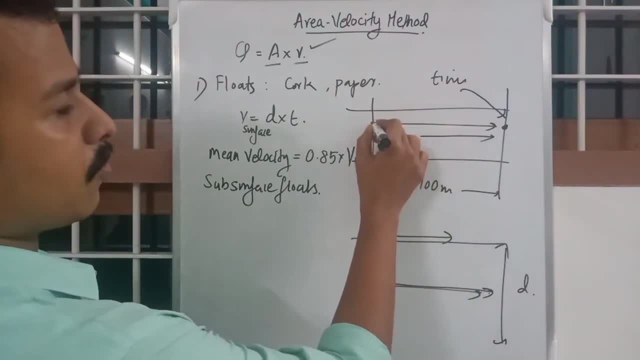 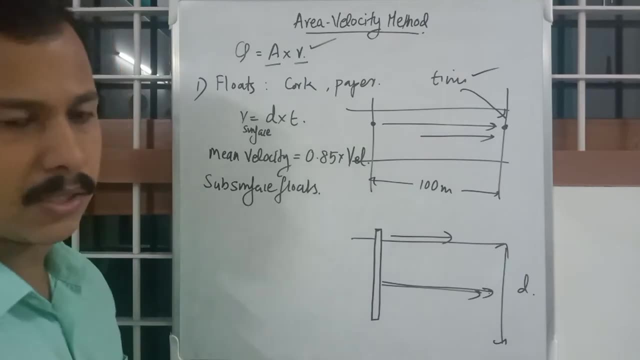 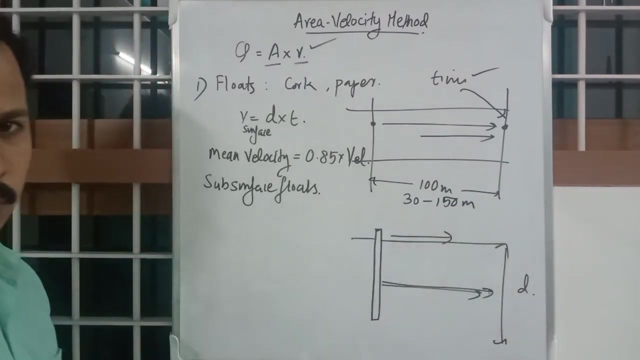 procedure is the same thing. you will start floating it, that road, at one point and will measure the time elapsed to reach a particular distance, and that distance is most probably 30 to 150 or 100 meters distance, usually ok- and this road. length of this road will be 0.94 mm. 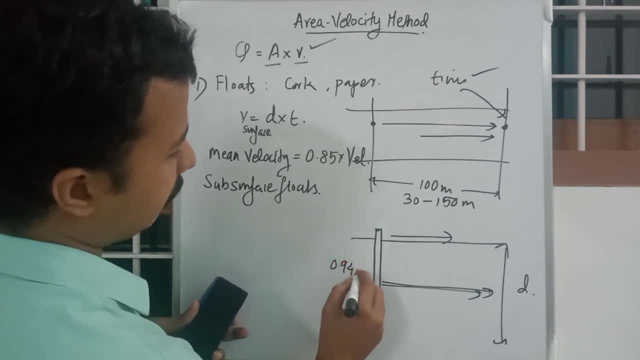 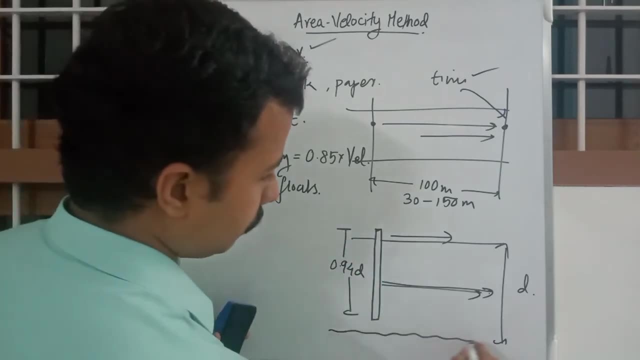 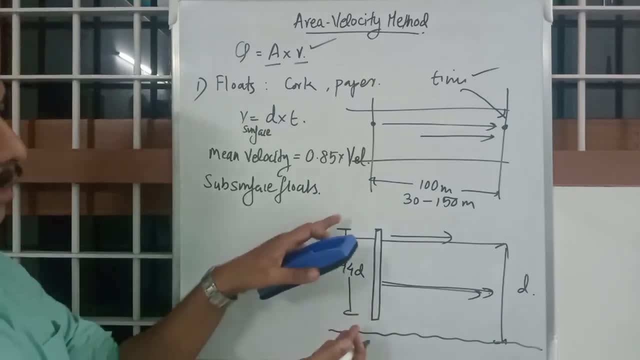 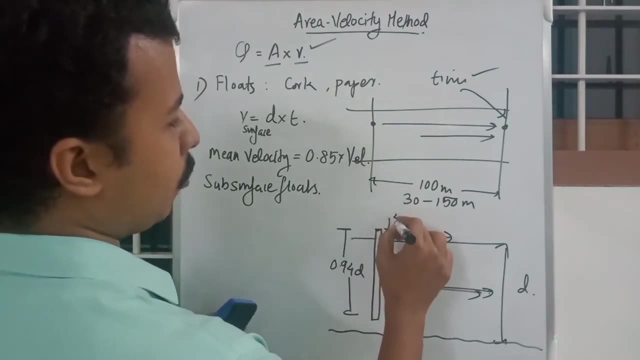 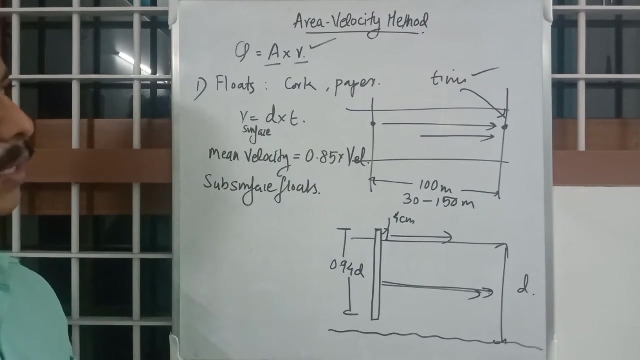 so Moin 94 D will be the length of this float road, okay, and approximately around four centimeter or five centimeter will be shown at the surface. okay, even if major portion is in under water, a four centimeter or five centimeter will be seen from the top. it will be floating above the surface and that measurement 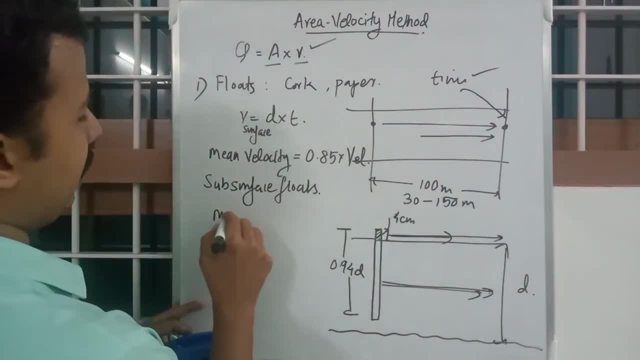 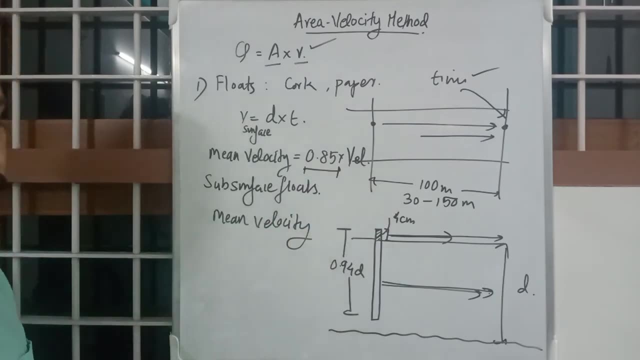 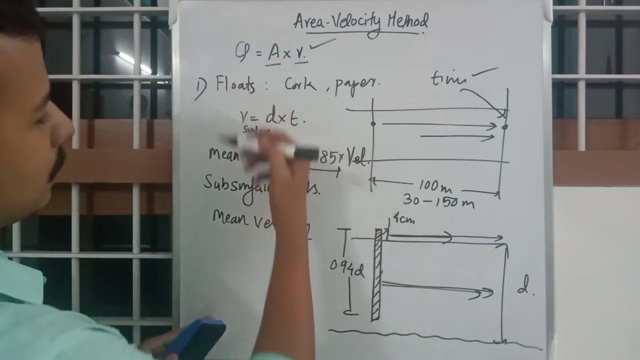 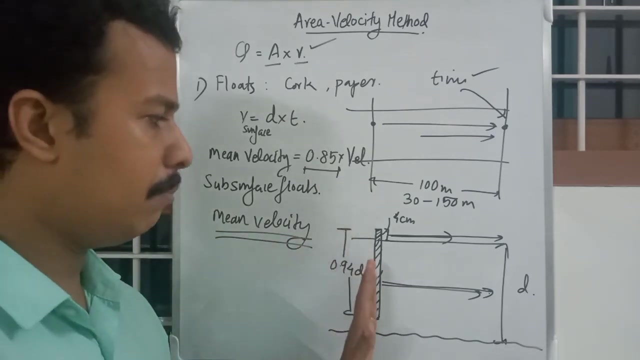 will give you directly mean velocity. there is no need to multiply 0.85 or any other factor. by measuring with subsurface floats you will get the direct value as mean velocity because it is already immersed into 90%. it is immersed in the inside the water, so the 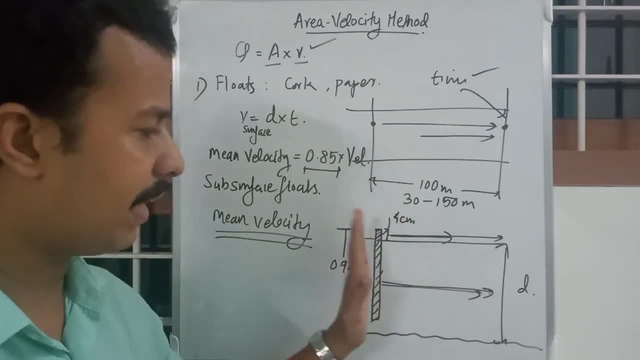 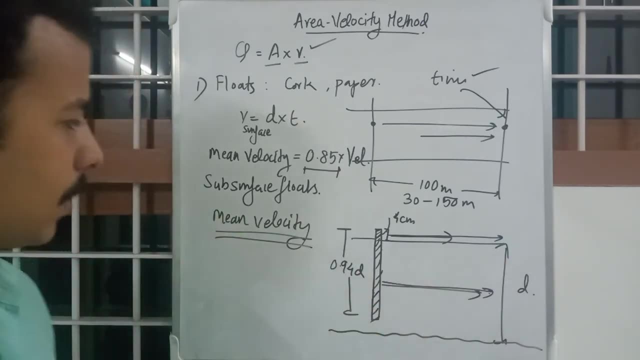 main current or main velocity stream. velocity will be directly affected by D, D, the float of this float, speed of this float. okay, so that is subsurface and surface floats okay, and the third one is measurement by instruments. mainly this second one: floats will be subsurface and 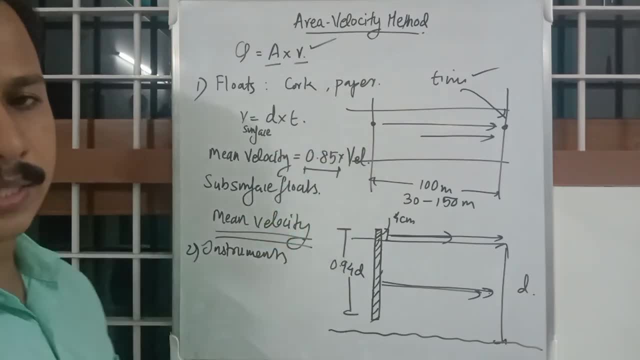 subsurface ports. second one: instruments- usually we use pitot tubes for the float- start to float and surface will float. that means this is zeroOH or primary kind of floating mode. packet is possible to get the measurement, the plant manager, as close as possible. this are the mes exaggerations. 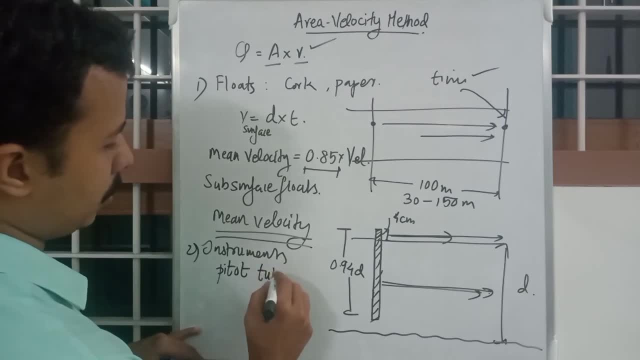 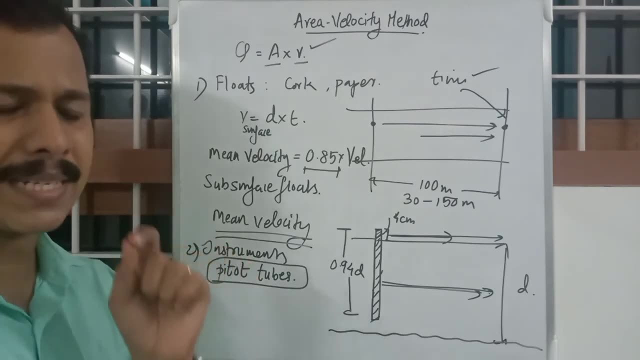 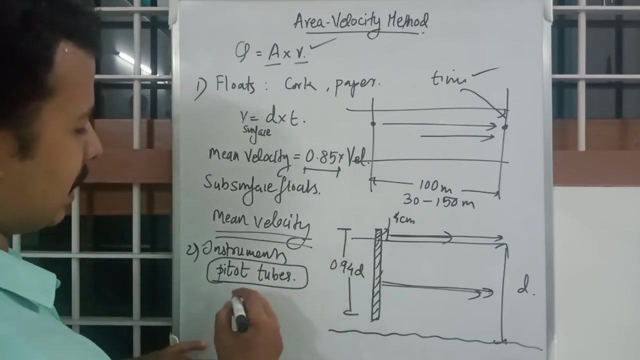 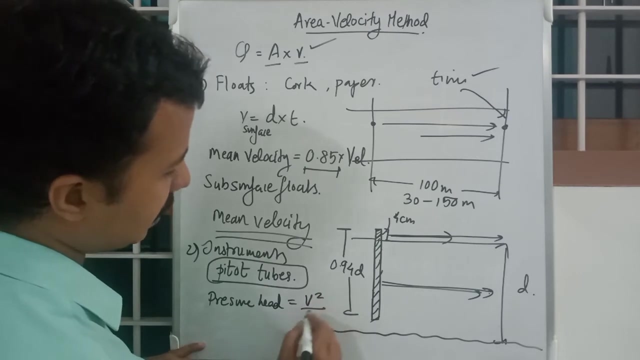 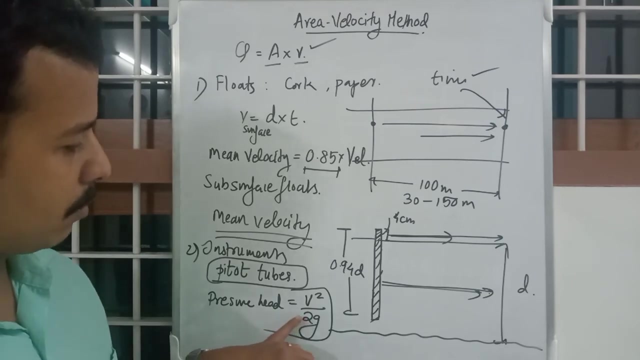 pitot tubes. this a very common instrument that is used to measure the velocity of water in pipes, closed sections, etc. but in here, if we use it, it will be measuring pressure head. pressure head, that is V square by 2g. okay, so pressure head of a flowing water is termed as V square by 2g, V being the 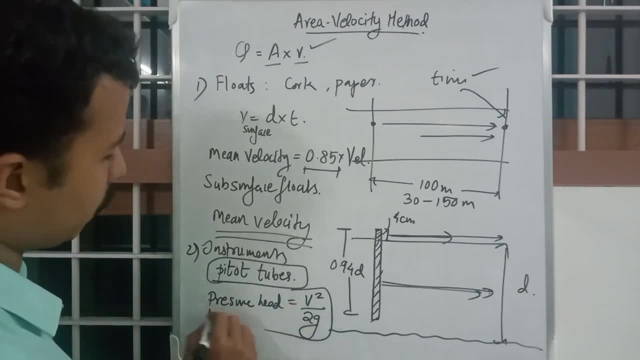 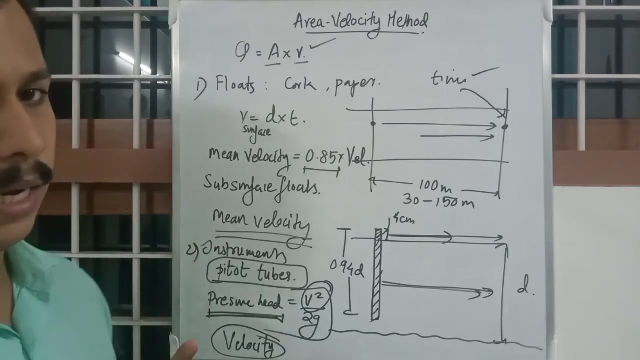 velocity and from this value, using pitot tube, you will get pressure head value and by equating that value you will get V velocity and that can be assumed as mean velocity. okay, so these two are the main used or commonly used methods. okay, so these two are the main used or commonly used methods. 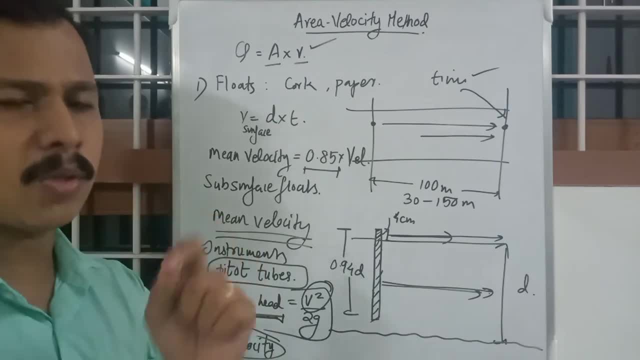 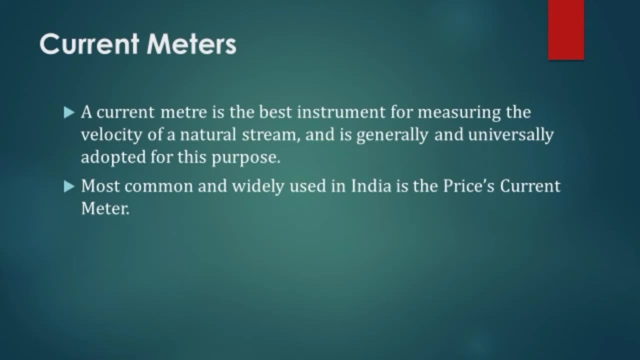 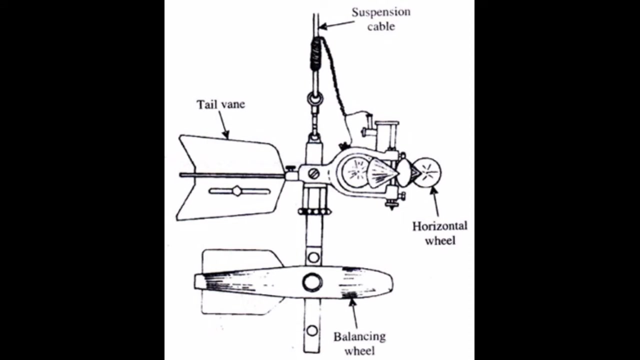 to find velocity. and the next, and the most common one, is current meter. so a current meter is the best instrument for measuring velocity of a natural stream and is generally and universally adopted for this purpose. the most common type is prices- current meter, and this is prices- current meter, and this will be 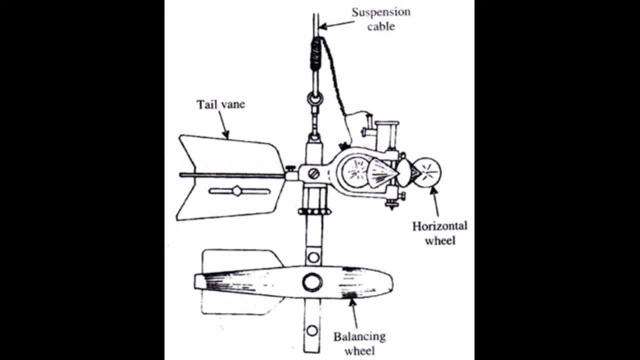 suspended by a suspension cable from the surface and will be immersed in the water. and be reminded, this figure is very important for you guys. okay, and the main and the most important part of current meter is the horizontal wheel, which will rotate in a vertical axis, as you can see in the figure that 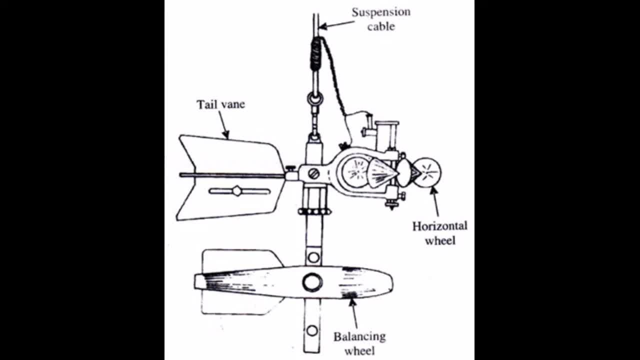 will act: half of the cups concave and the other half half convex, while in a current flow, current of our considering stream, there will be a tail vane and a in the behind so that the position of current meter aligns with the current or flow of water, and at the bottom there will be a balancing wheel so that it does. 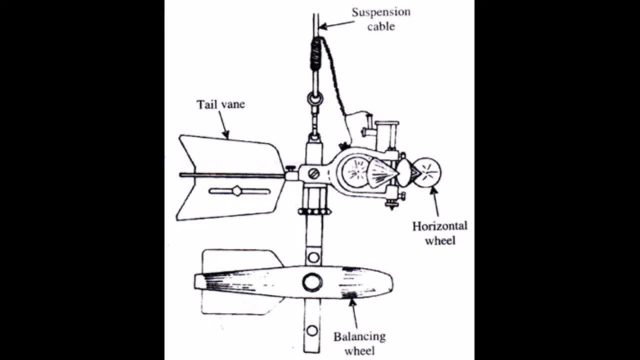 not topple or tilt in the water, so that has to keep it vertical. okay, so we have already seen similar instruments for measuring wind velocity. there is live, there will be a rotating horizontal wheel and there will be tail vane for adjusting by itself. so the components- suspension, cable, horizontal wheel, balancing wheel, tail- 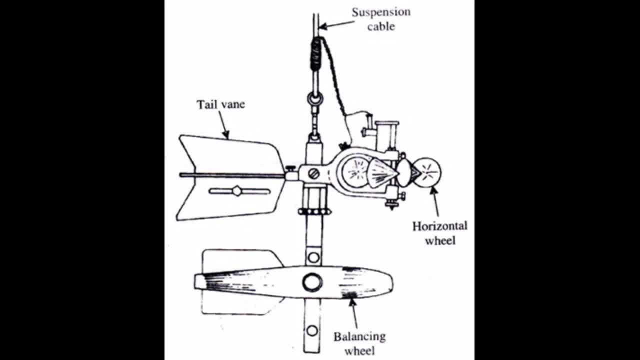 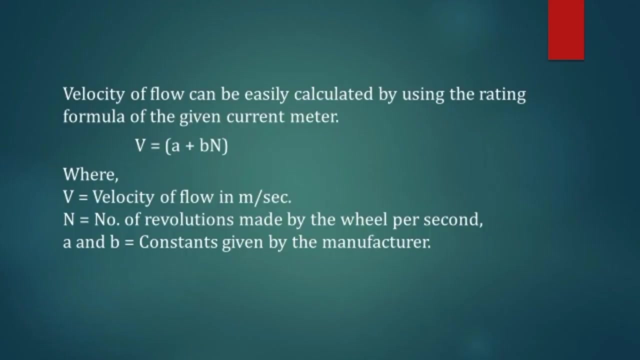 vane, and in addition to that, there will be a path that will count the rotation of this horizontal wheel and that will be record as n. the machine by itself will count how many times this wheel is rotated by the flow of stream. okay, and the velocity of flow can be easily calculated by this.